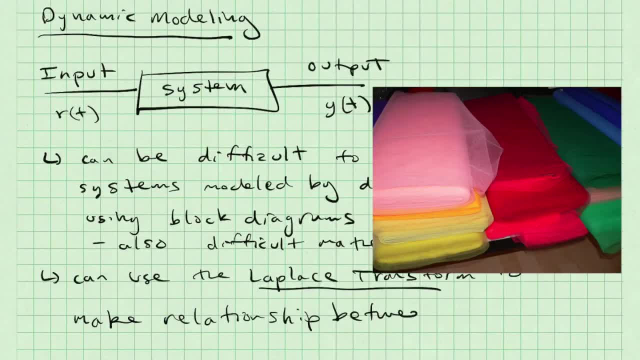 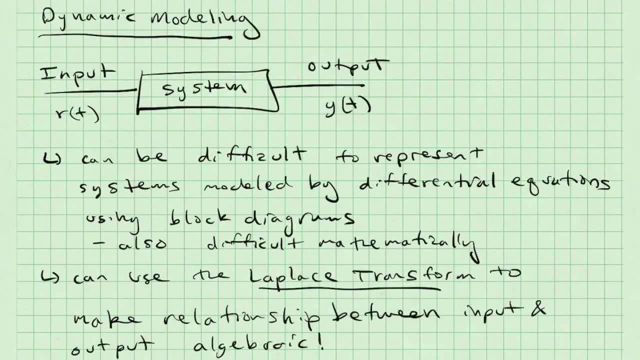 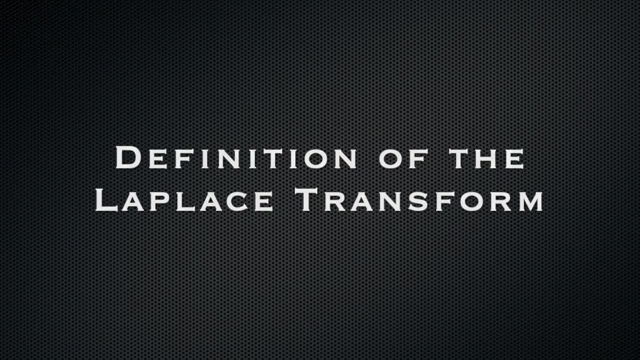 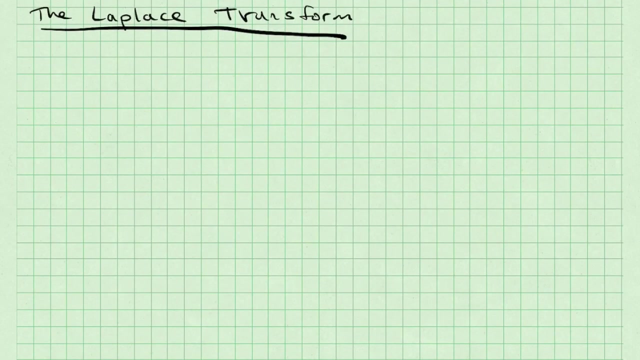 So one tool we can use is the Laplace transform. This tool allows us to make the relationship between the input and the output of the system algebraic, And a lot more of us are comfortable with algebra than are comfortable with differential equations. Let's introduce the Laplace transform with its definition. The Laplace transform of a time domain, function f of t, is: 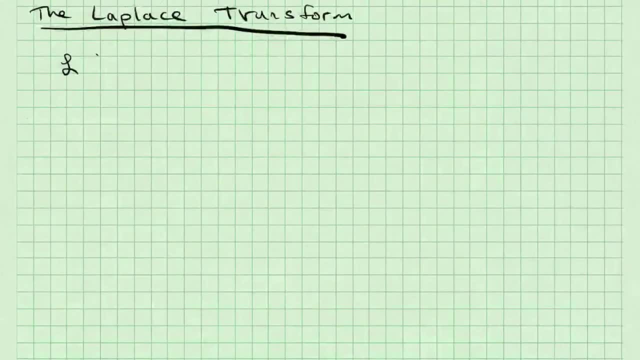 represented by using a squiggly L, And this Laplace transform is equal to capital F of s, a function of s. We use the capital letter to distinguish between time domain, which is lowercase, and Laplace domain, which is uppercase. This is equal to the integral from zero minus, or the instant right before zero. 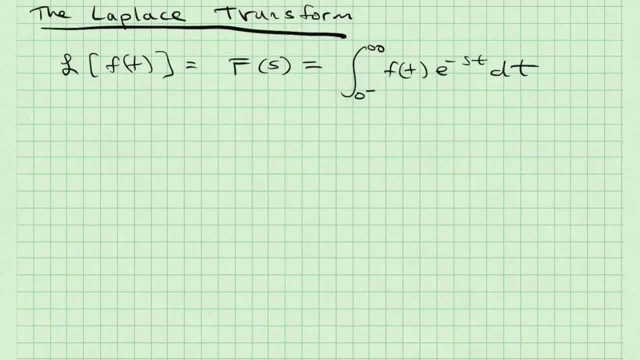 to infinity, of f, of t, e to the minus st, dt. The variable s is a complex variable which has a value: sigma plus j, omega. Sigma is the real part of s and omega is the imaginary part. I noticed that, since the integral is over t and takes place over the range of all positive values of t, that I'm eliminating t. 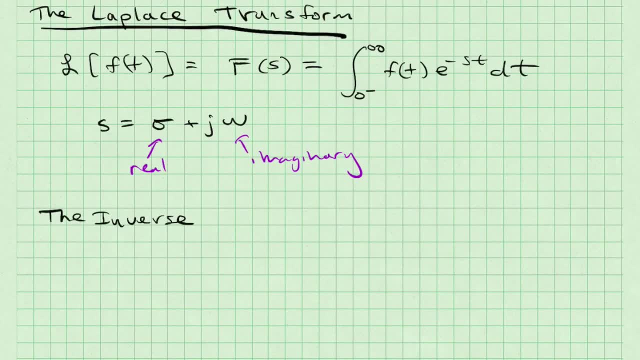 from my expression, I'm left with the variable s. On the other hand, I can take the inverse Laplace transform, which is represented as again that squiggly L with an inverse of the Laplace domain function, big F of s and it's equal to 1 over 2. pi j integral from sigma minus j, infinity to sigma. 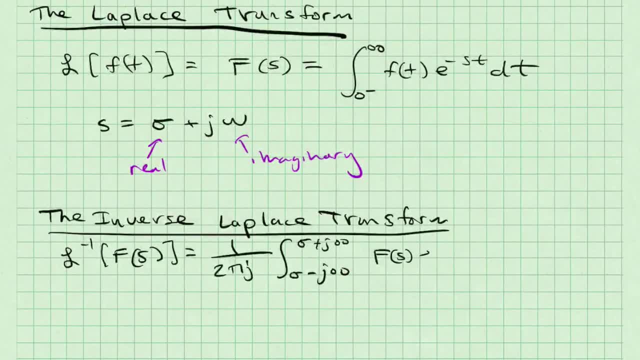 plus j infinity of f of s, e to the st ds Which I represent as f of t, u of t. More on that in a second, Integrating over all possible values of s, I eliminate s from the expression and I get f of t. Now, what is? u of t? u of t, which is called the unit step? 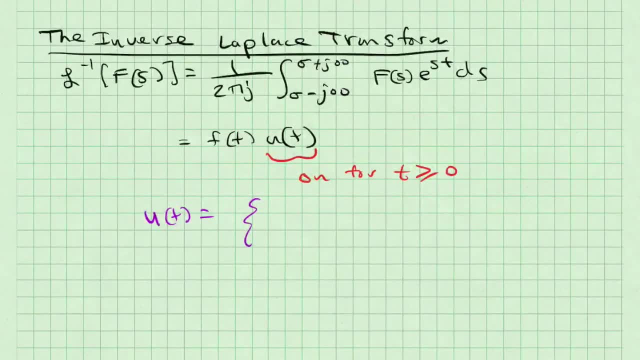 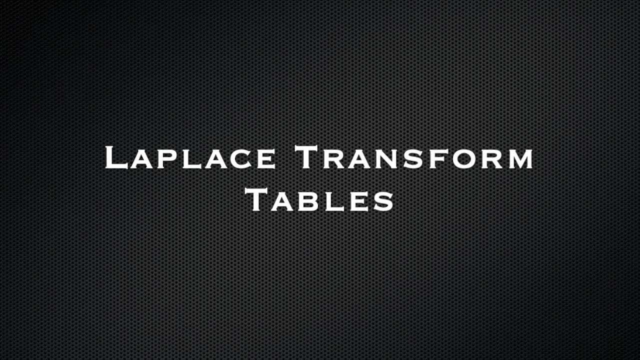 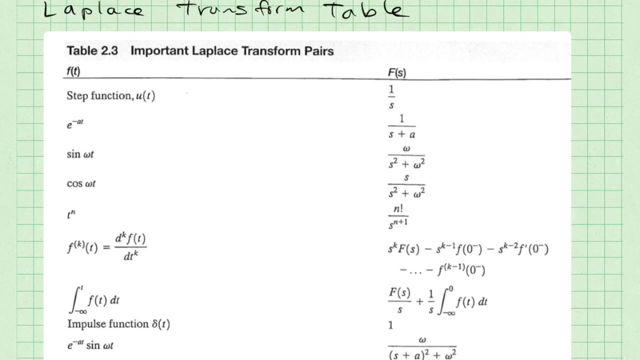 is equal to 1 for t greater than or equal to zero and zero for t less than zero, It means that this function is on for t greater than or equal to zero. Many functions have established Laplace transforms. What I'm going to do is to point to the important ones for control systems on this table. 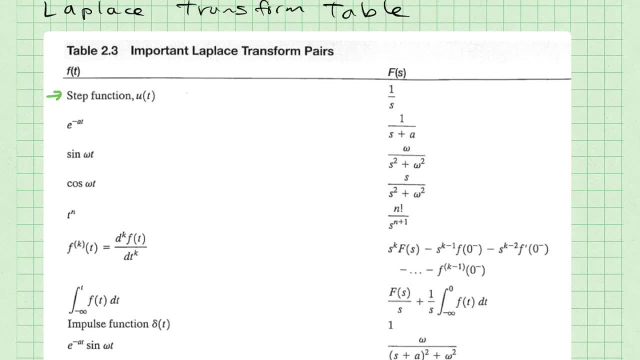 The step function u of t which we discussed has a Laplace transform of 1 over s. e to the minus a t is very important because many of the characteristic modes in differential equations can be represented as e to the minus a t. 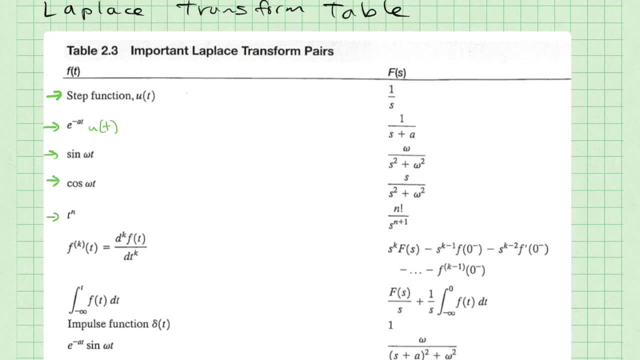 Now, strictly speaking, for most of these important pairs, there should be a u of t appended to the end: Sine, omega t, cosine, omega t, t to the n. all should be appended by u of t. These are all important. 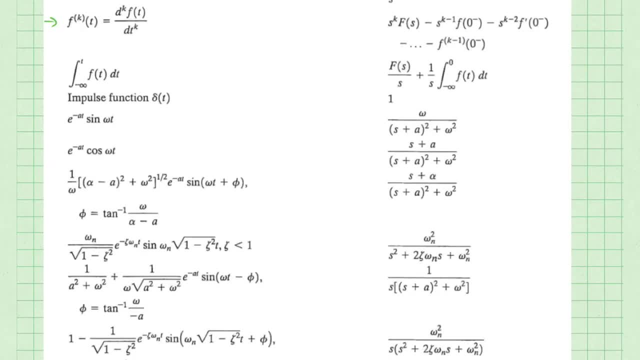 The derivative is also important. The integral, the impulse, which needs no extra u of t And e to the minus a t, both sine of t and cosine of t. These are the really, really important transforms that you might want to use in control systems that we will make use of throughout the rest of these lectures I'm intending to do. 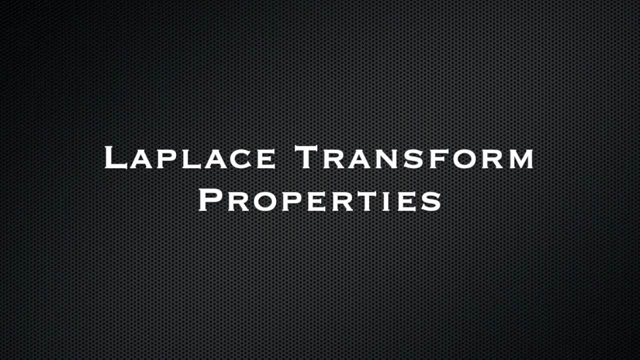 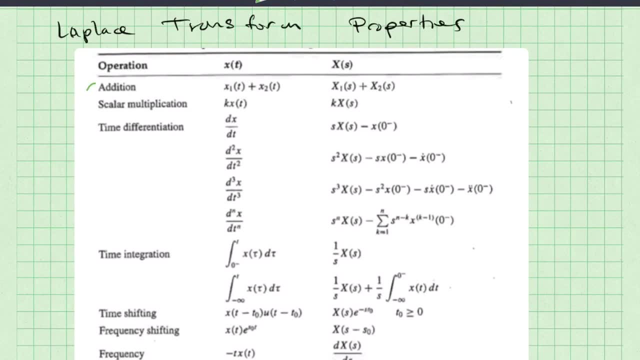 The Laplace transform has a number of very nice properties. The first two: addition and scalar multiplication. multiplication actually mean that the Laplace transform is a linear operation. It says that if I multiply the time domain function by a scalar k, that the Laplace domain function is. 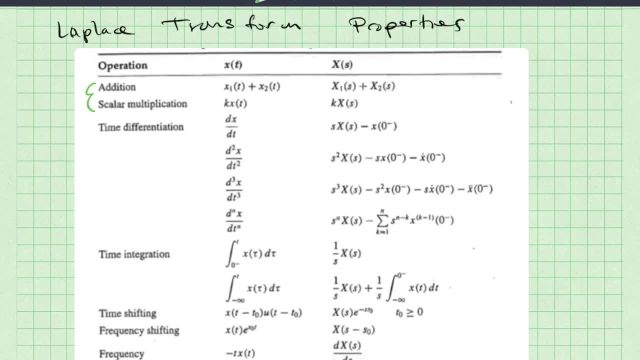 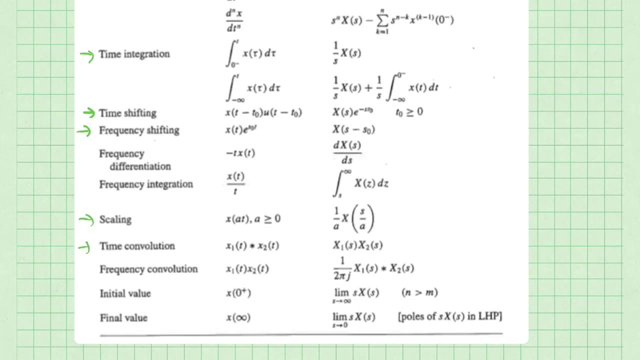 also multiplied by that same scalar. And if I add two time domain functions together, their Laplace transform is the sum of the Laplace transform of each of them taken individually. Other important properties are time differentiation, time integration, time shifting, frequency shifting, scaling, time convolution, initial value and final value theorem. 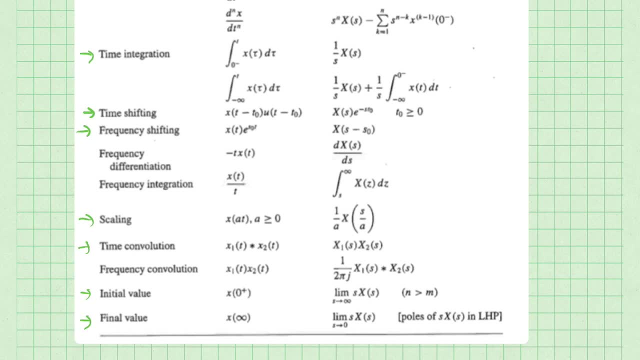 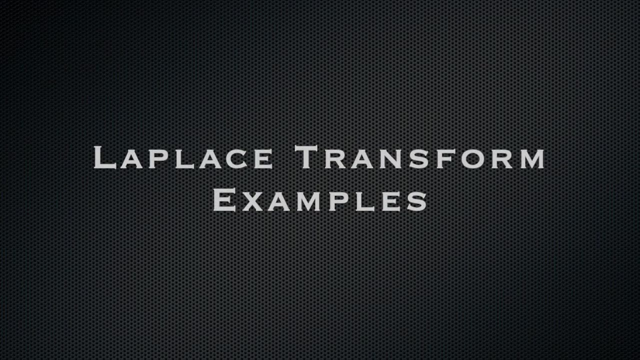 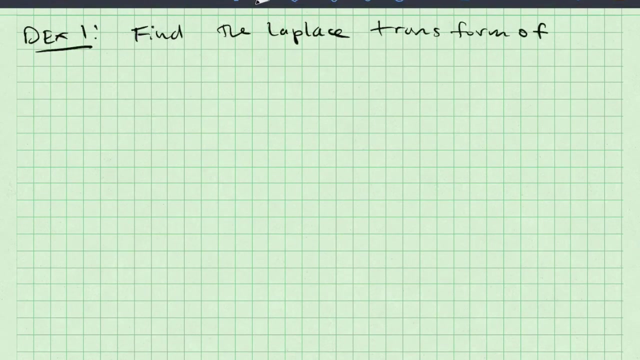 Some of these other properties, while useful, don't often see a lot of mention in control systems. Okay, I would like to apply some of what we've learned about to some examples. In the first example, I'd like to find the Laplace transform of a time domain function f of t. 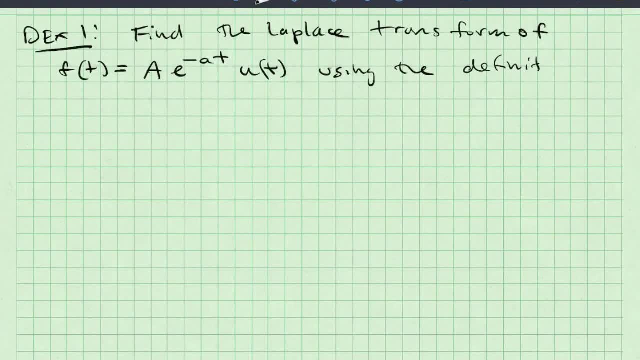 which is equal to a e to the minus at u of t, And I want to do so using the definition of the Laplace transform. To start with, I'm going to write that definition down, Then I'm going to plug in the Laplace transform of a time domain function f of t, which is equal to a e to the 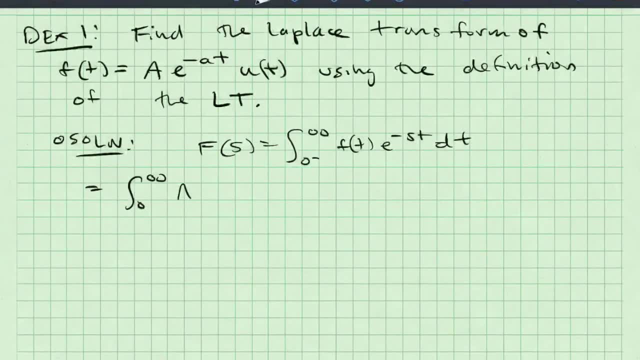 minus at u of t And I'm going to plug in the value of f of t So I get the integral from 0 to infinity of a, e to the minus at e to the minus st dt. a is a constant, so I can pull it out front. 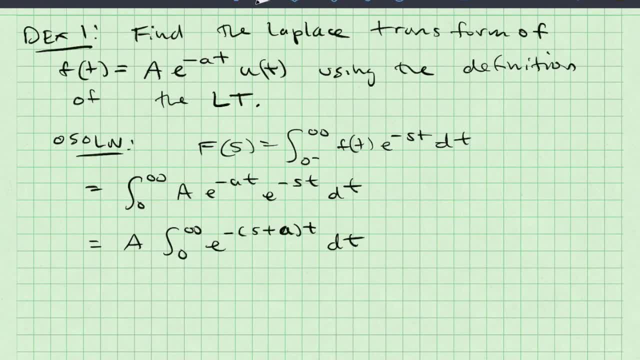 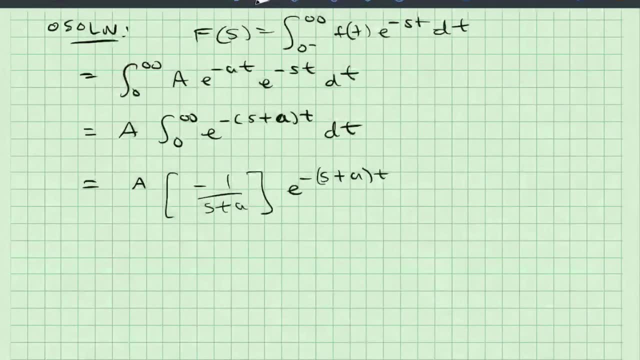 and I can take those two exponentials and I can mush them together. Executing this integral, I'll get a multiplied by negative, 1 over s plus a e to the minus s plus at, And that whole thing is going to be evaluated between 0 and infinity. Taking e to the negative, infinity is 0.. Taking e: